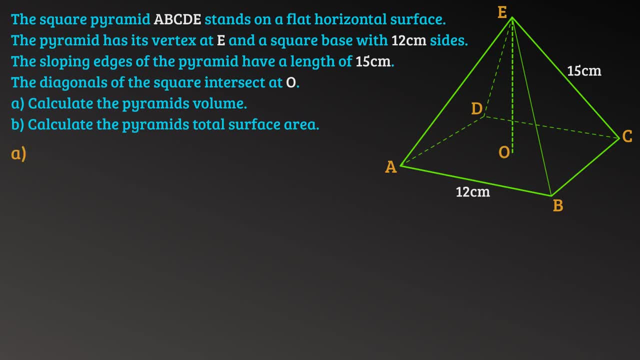 And we know the middle of the square base is O, as the diagonals intersect there. Now we're asked to find the volume, for which we'll need this equation, where volume is a third base area times height. Now the base area should be easy to find, it's just the area of a square, but we need to find the height here. 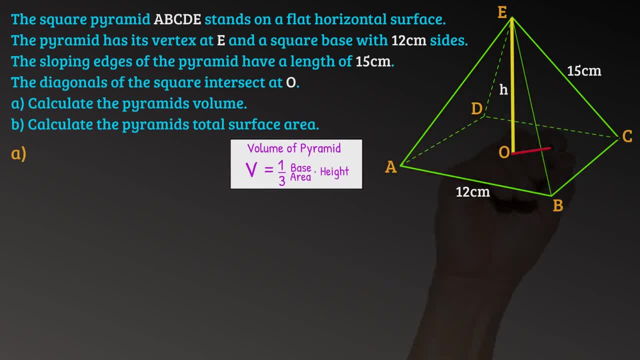 Now, if we make this into a triangle to the corner of the square here- and I'll draw this triangle below to make it clearer- we already have the hypotenuse, which is 15cm long. We want to find the height, but first we need to find OC. 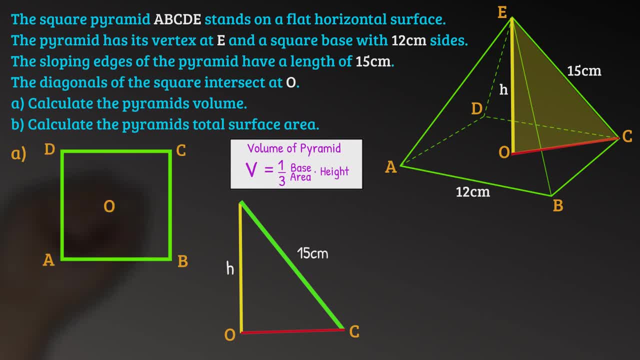 which is the base, which is in red. So first let's draw the base of the pyramid and draw in the line OC. Now we know the base of the pyramid is a square with sides of 12cm long, So we can draw a right angled triangle here where OC is the hypotenuse. 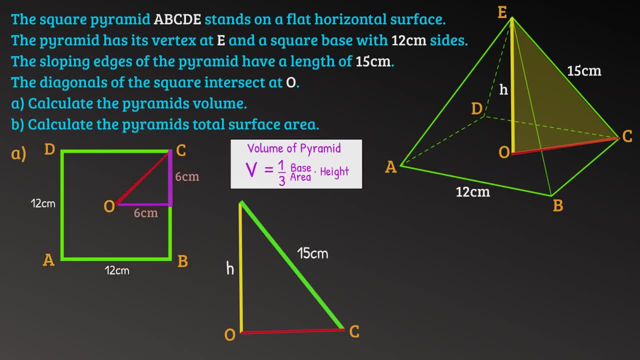 and then we know the other two sides are both 6cm long And then we can use Pythagoras to work out OC. So OC squared is going to be 6 squared plus 6 squared, which works out as the square root of 72.. 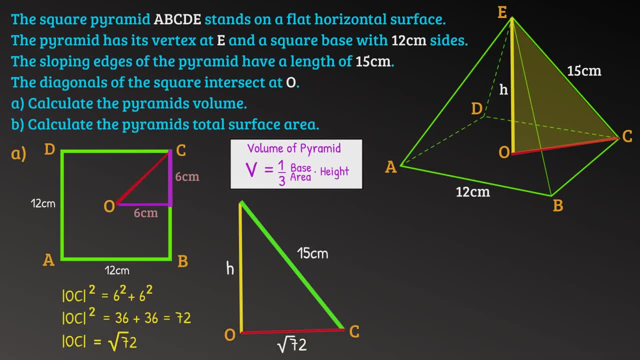 So now we've worked out the length of the base of this triangle, we can work out the height also using Pythagoras. So we have: 15 squared is equal to H squared plus the square root of 72 squared. Well, the square of a square root is just the number. 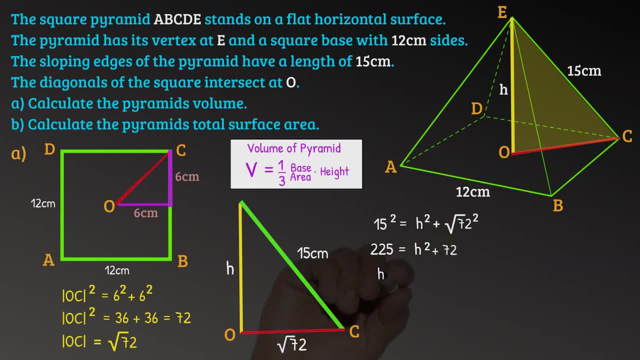 so we have: 225 is equal to H squared plus 72.. So we can work out the height as the square root of 153, or 12.37cm. The base area is just the area of a 12cm sided square. 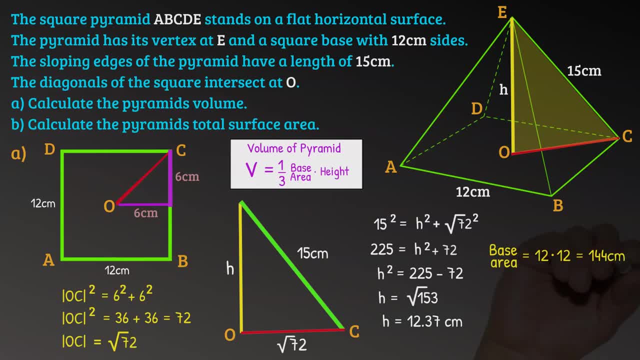 which is just 12 times 12, or 144cm squared. So, using the formula, the volume is 144 times 12.37 divided by 3,, which is 593.76cm3.. In part B we have to calculate the total surface area of the pyramid.